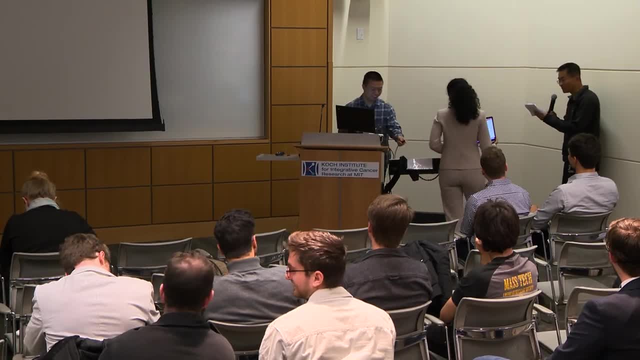 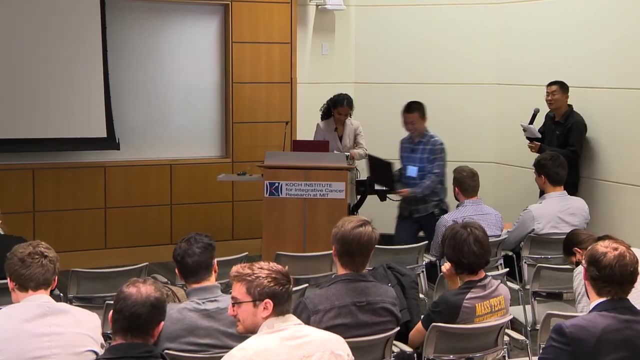 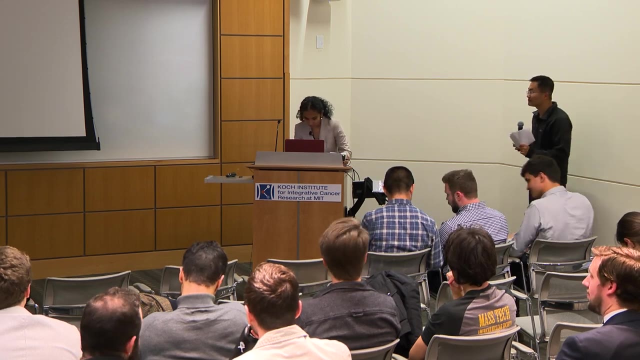 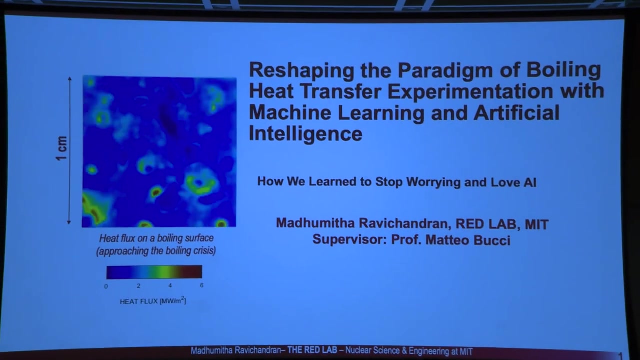 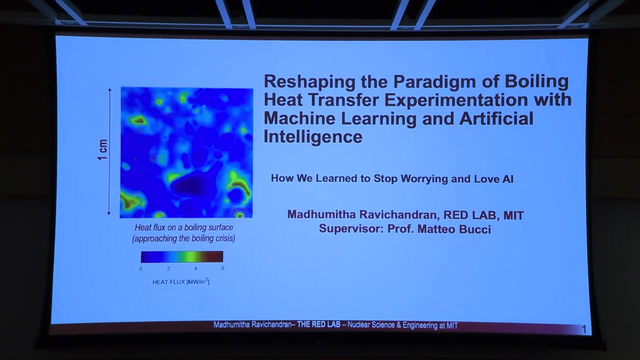 Our next speaker is Madhumisa Ravichandran and she will talk about on the using of machine learning on hydrodynamics. Thank you for the introduction, Professor Lee, And hello everyone. Let's first start by watching this video and spend a moment on it. It's. 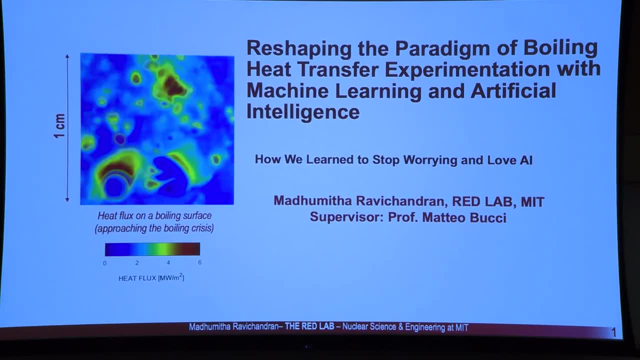 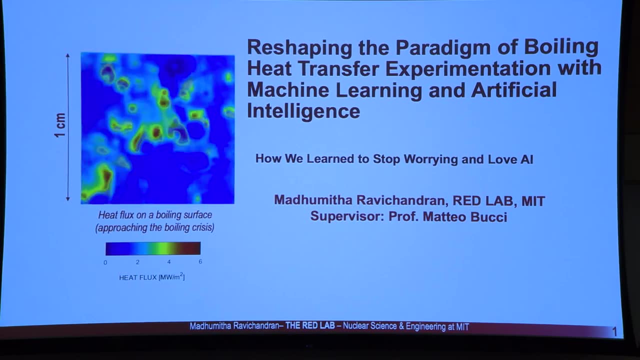 colorful and it's puzzling. And I say it's puzzling because I'm launching a lot of data at you. To be precise, it's about a gigabyte of data that I've launched And it's nice to watch but almost again impossible to process as we see it. And what if I told you: 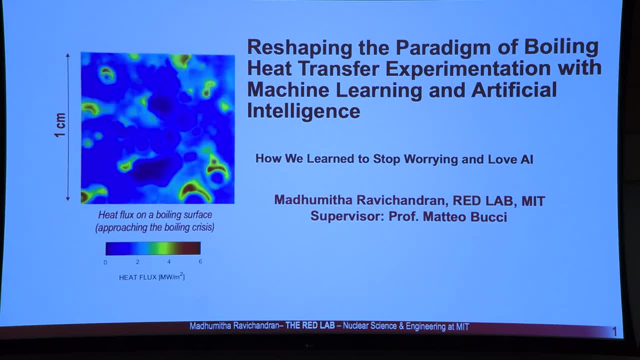 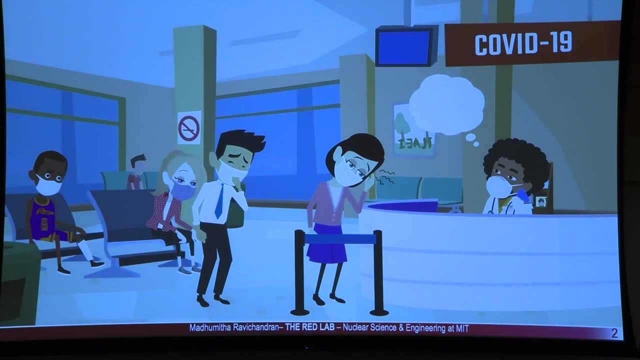 that you could uncover a lot of mysteries that drive nuclear reactors. if you understand how much I understood this video, My lab mates and I took the plunge. We were motivated enough, so we sat and binged on these videos during the pandemic, while many took to Netflix. 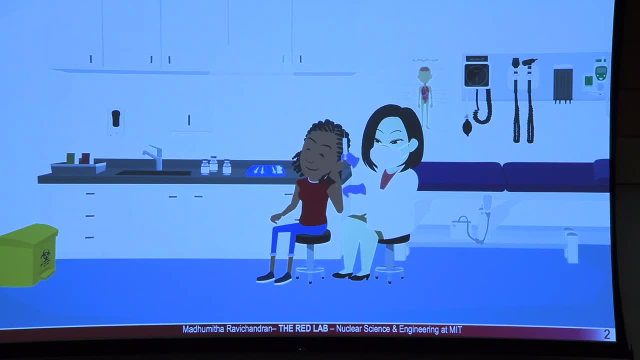 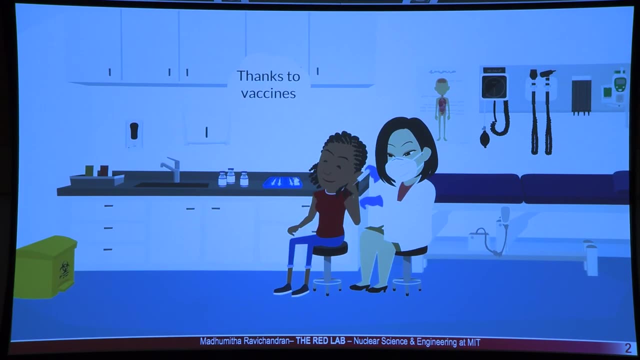 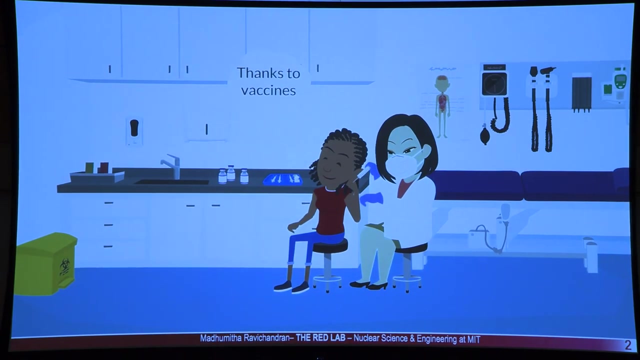 The pandemic has affected us all and we've been thinking about it a lot. Situations may have been worse if not for the timely development and administration of vaccines, And historically, vaccines used to take several years to develop and synthesize and test multiple nuclear reactors. 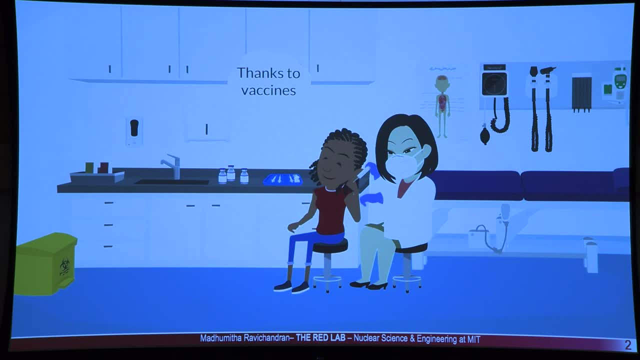 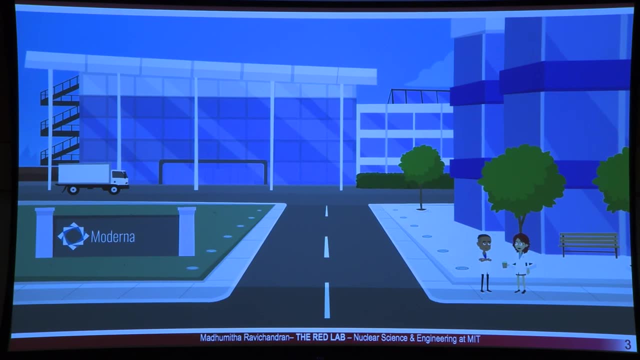 But when a diagnostic measurement was done, the diagnosis was that a'mrna could be ready at a faster rate and that it could be delivered. But in the case of the COVID-19 vaccine, the mRNA vaccine developed after a few months, with the onset of the disease And out of 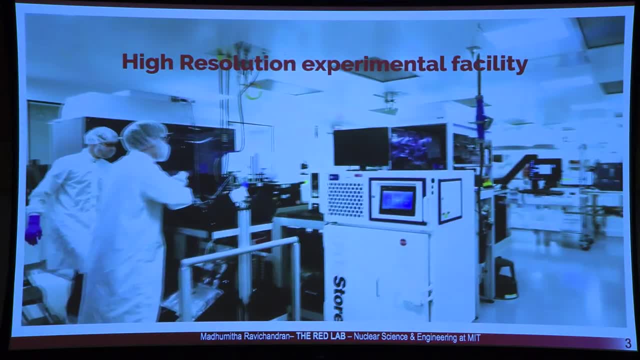 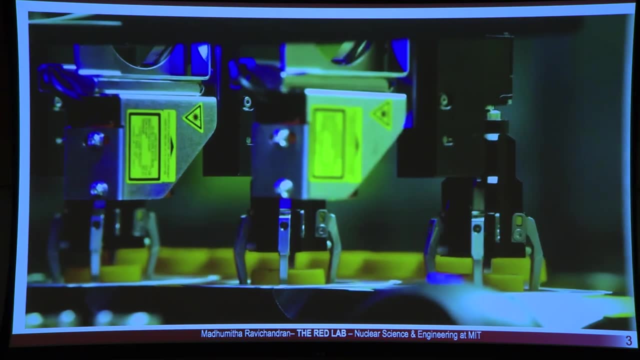 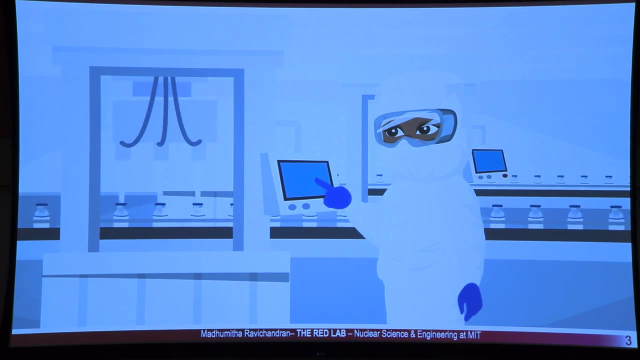 many contributors. two tech contributors have been significant. One is high-resolution experimentation And the other was the automation of whole process workflow itself In synthesizing and in studying our different nucleic acid chains and these. this combination is revolutionizing the way we see our experiments and test of experiments in 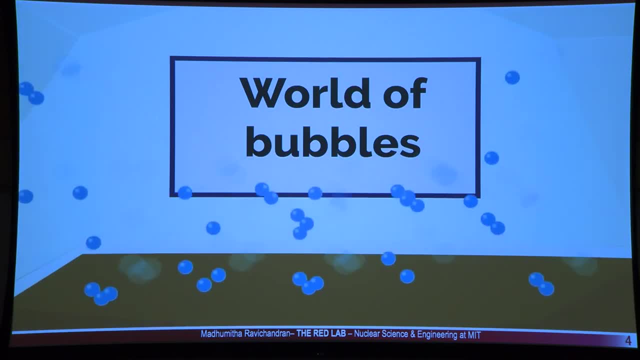 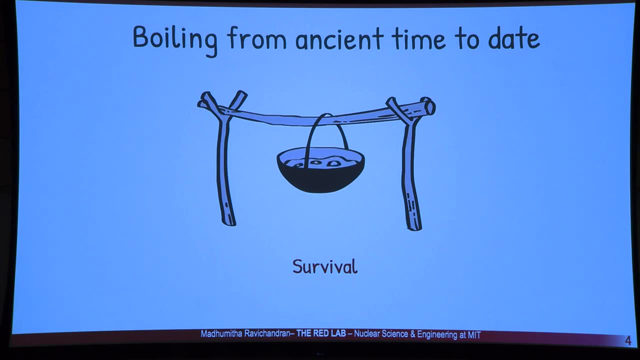 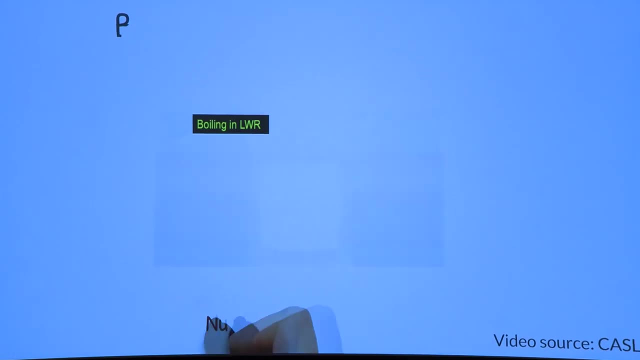 many fields, and that's my focus, but in the field of bubbles and boiling heat transfer- and boiling heat transfer has been of significance to us from a very long time, come on. we've all survived this long, and we also build efficient energy systems that use boiling heat transfer, and I'm talking about 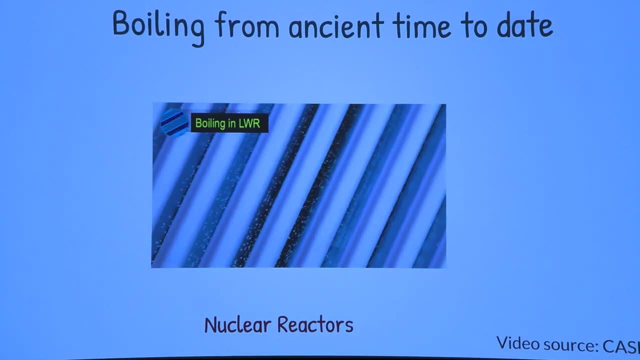 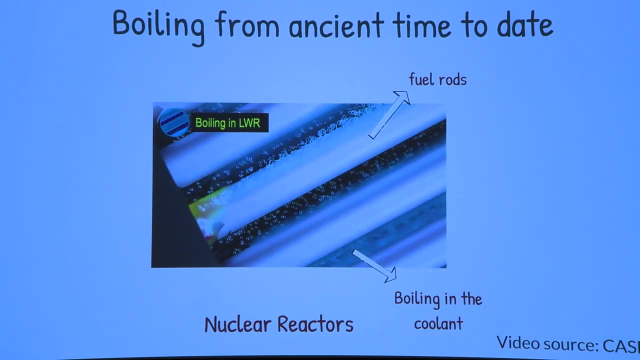 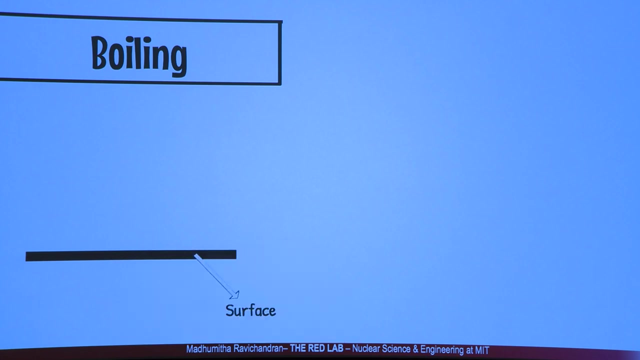 light-water reactors. here you're looking at the fuel rodlets that are cooled by a few by fluid, and you can also observe bubbles that cool the fuel rods in light-water reactors. and now thinking about formation of bubbles, let's first see what boiling is. imagine there's a surface that gets heated and 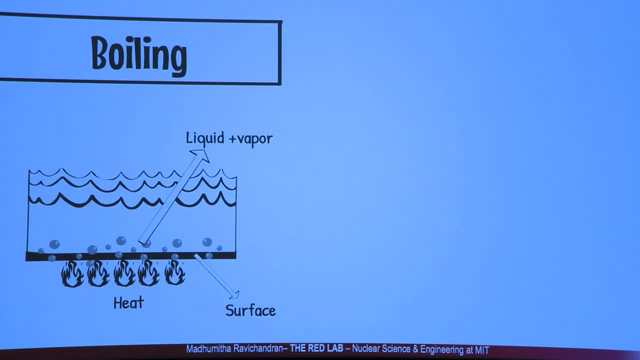 there's fluid either flowing or it could even be stagnant, as I've shown here. as the fluid gets heated, bubbles start forming and remove heat from the surface, and that's what we call the boiling heat transfer. and that's what we call the boiling heat transfer and that's the simplest definition of boiling that I. 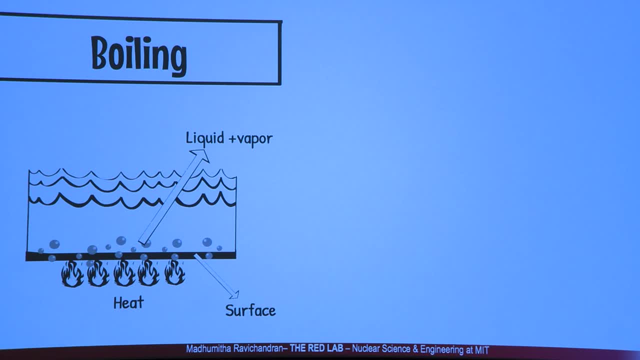 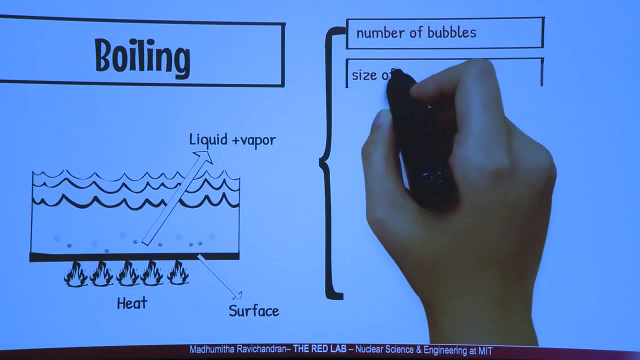 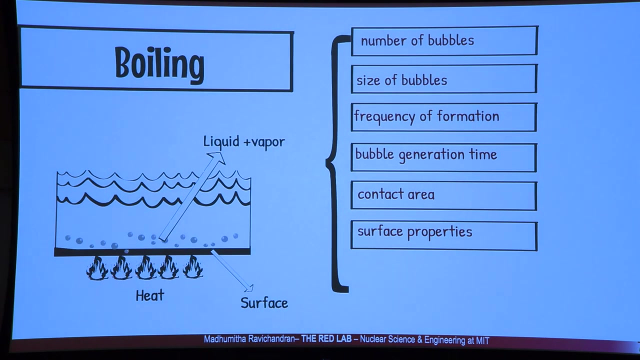 could ever give you, and because there are multiple factors that drive the heat transferred when we start seeing bubbles, and these could range anywhere between bubble features, like the number of bubbles or the size of bubbles we form, or it could even be surface driven, like the surface roughness or the 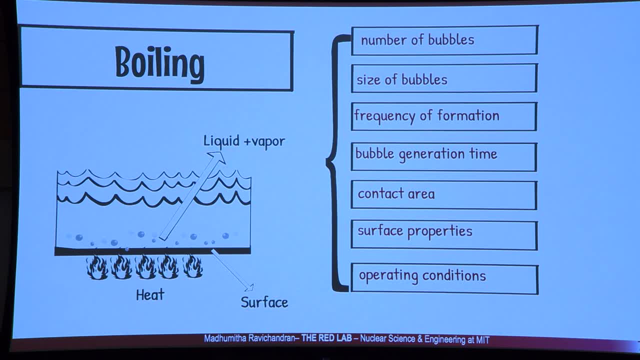 wettability of the surface. and there are again operating conditions that severely impact the boiling heat transferred, like the temperature or the pressure of operation. apart from these, there is a phase in boiling that completely shatters or transforms the boiling heat transferred and makes boiling almost unusable. and 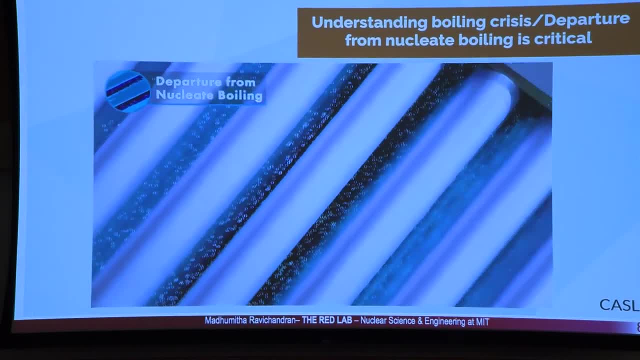 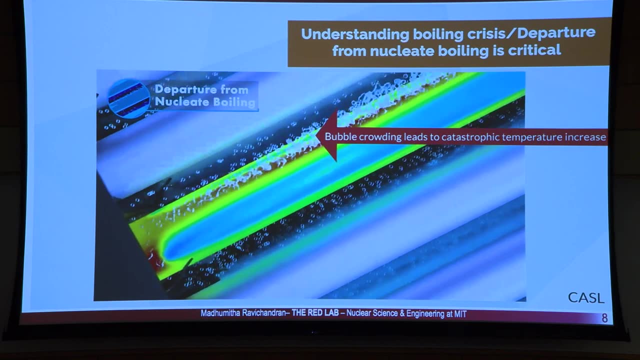 that let's say, let's look back at the same video. now there are bubbles that you see, but let's see there's a sudden power surge that could lead to an over formation and accumulation of bubbles and we may not be able to remove them as fast as they're formed and that could lead to sudden and rapid temperature. 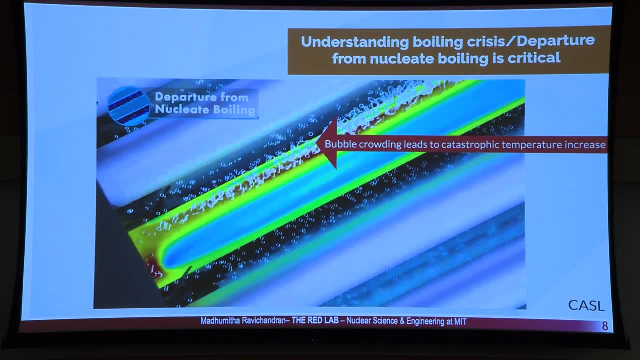 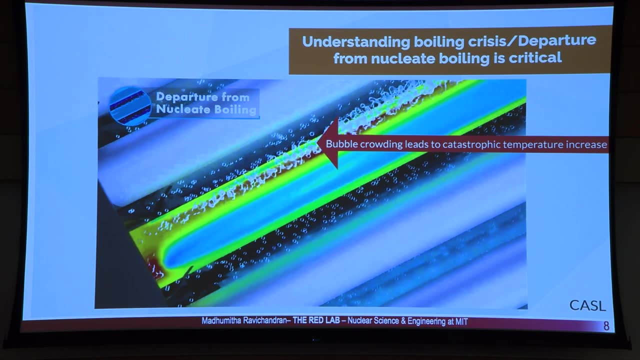 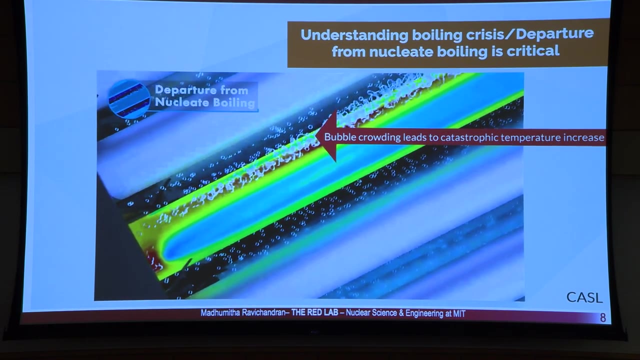 spikes and- And this could be catastrophic for a reactor, because the fuel rod could melt or we could go into any unforeseen catastrophe- And the Nuclear Regulatory Commission lays stringent limits on the operation of nuclear reactors so as to never see the boiling crisis. So that's what this is: the boiling crisis, or we'll also, I'm going to call it the departure. 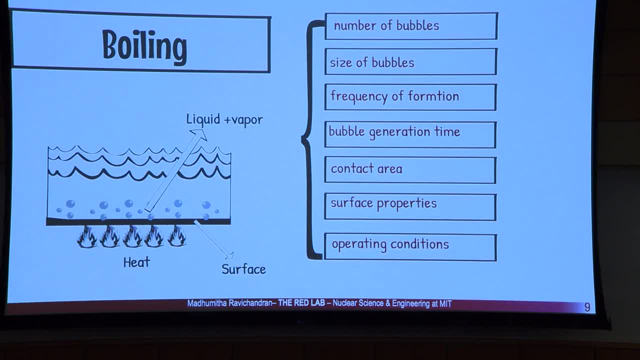 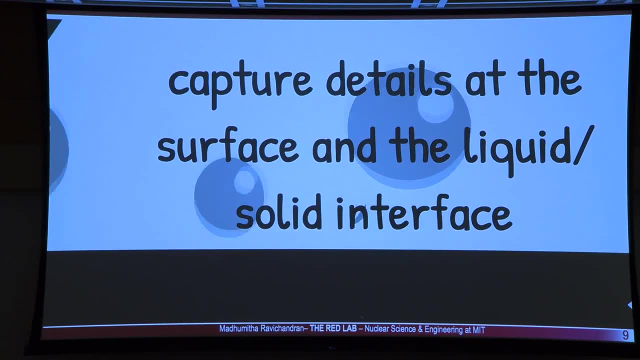 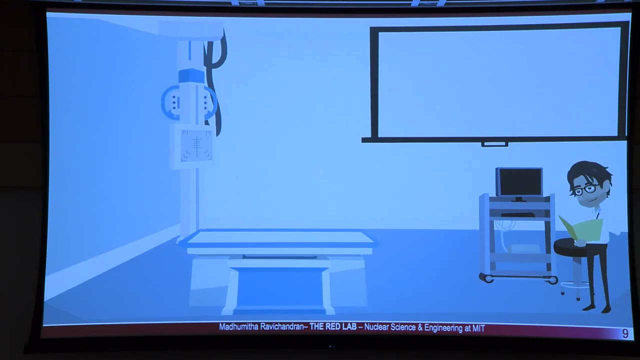 from nuclear boiling as well here, And scientists have spent decades trying to zoom in to the boiling process and see what happens at the bubble level, to quantify the boiling heat transfer accurately and also to see what happens during the boiling crisis. And now we have been able to accomplish that in our lab by building high resolution diagnostics. 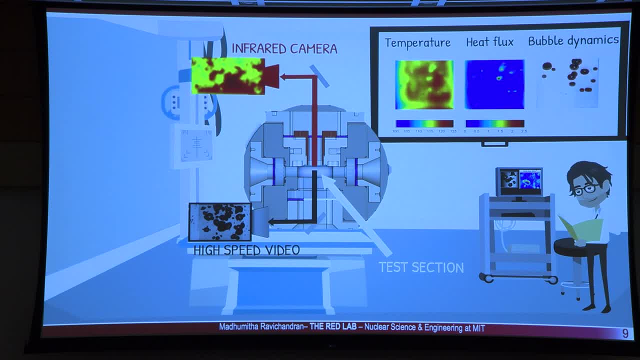 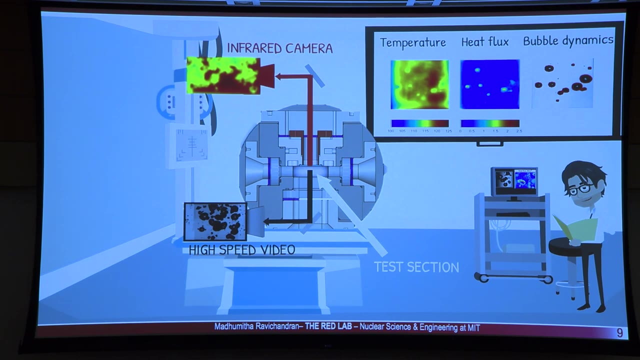 that my past lab mates have developed. So now we have our experimental setup where we run our experiments, but we can accurately track what happens on the surface as we run experiments. So we have an infrared camera. That's a high resolution camera That records all the temperature fluctuations as bubbles form and nucleate. 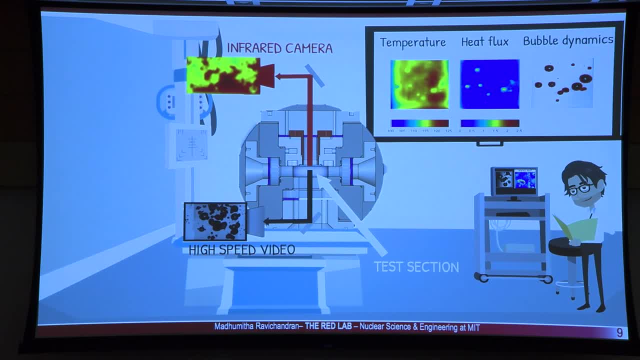 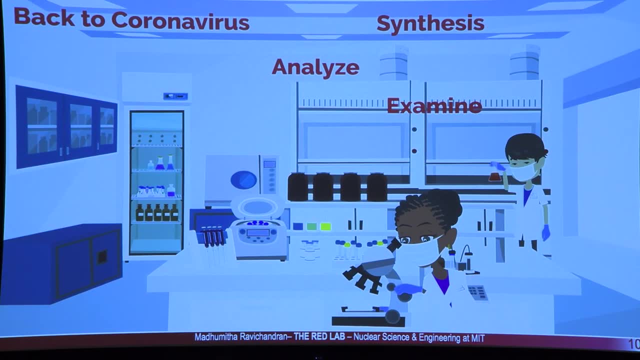 And we also combine this with a video camera that records all the bubble interactions that we need to visualize. But, again, similar to vaccine development, running boiling experiments is a multi-stage process And it also requires the to build. so, to build robust models, we need to run tests. 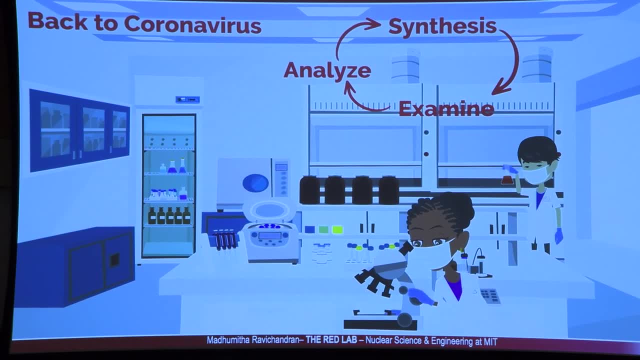 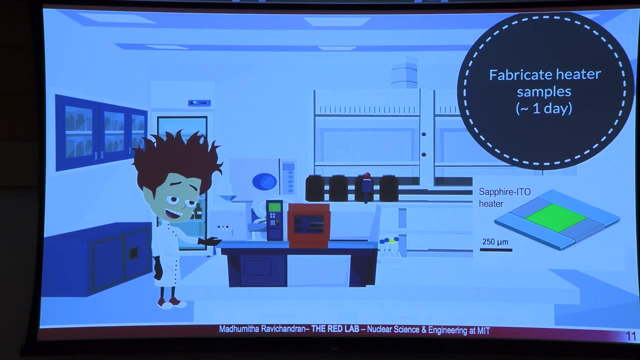 for multiple different surfaces And we have to test for different conditions. So for that we start out by fabricating a sample, And that takes us about a day to complete. And once this is fabricated we set it up into our experiment and run the whole experiment. 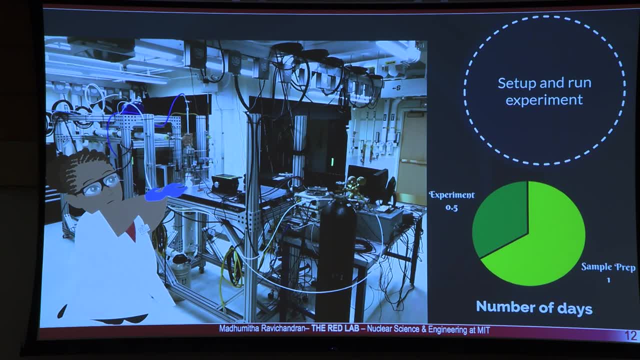 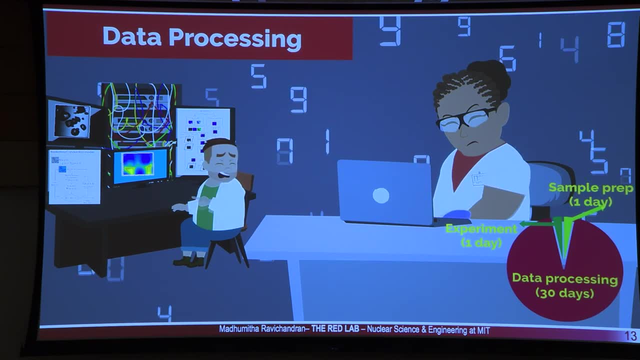 Let's say that takes us about half a day, or say one day, for now. Once we've run our experiment we acquire a lot of data that we process. So I'm not really exaggerating here when I say that it takes us a day or less than a. 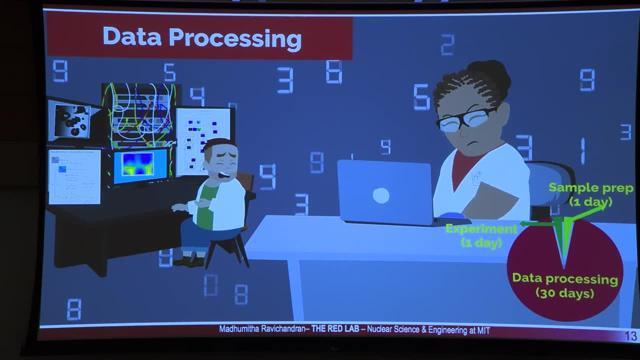 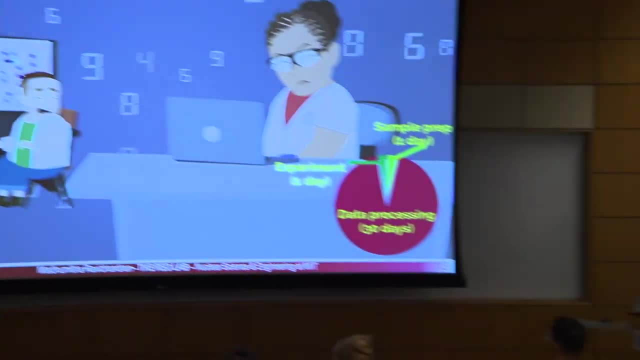 day to run an experiment, But it takes us about 30 days to process this data Because the post-processing is not really straightforward And we employ a lot of different techniques And we also have to visually keep looking at bubbles and quantify the process that happens. 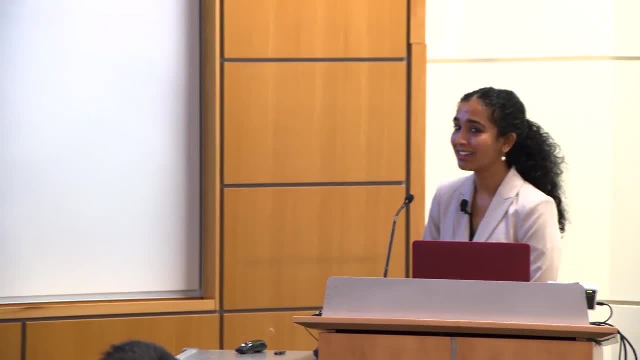 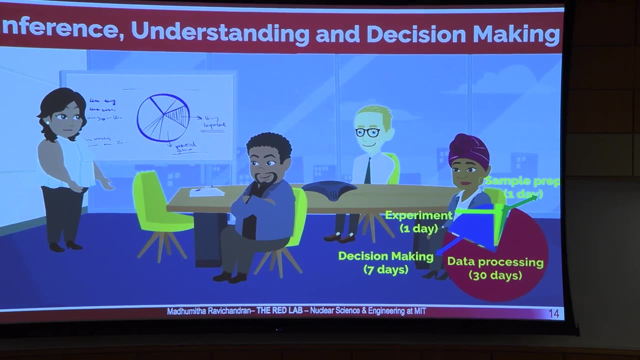 And once we have these results, we sit together and discuss the implications of the experiment that we just finished, to chart out the next course of experiment, or fabricate a new surface, or we decide the next course of action basically. So this is the whole process. 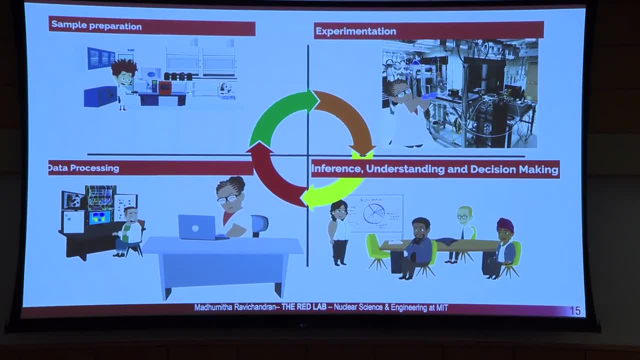 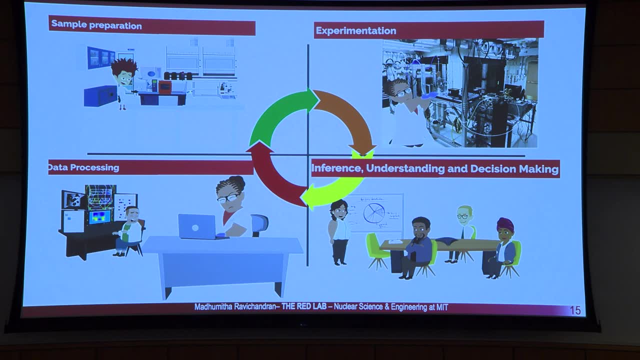 And what we do is that we repeat several times to process data and to run multiple experiments, And we run experiments on multiple different surfaces, on different conditions, And we also repeat some experiments just to make sure that we get the same results every time. Here we started thinking that there's so much of human intervention that is required to 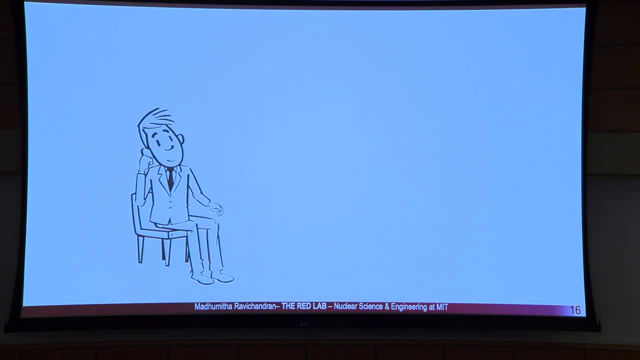 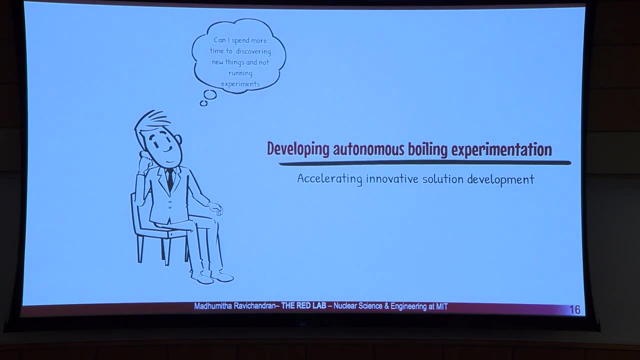 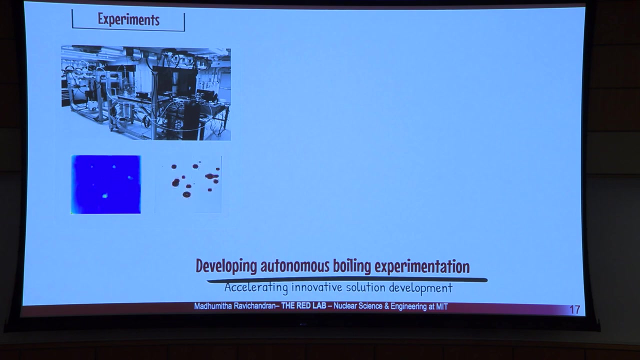 set up and run our experiments and process data. And, as anyone would wonder, And especially as researchers, We like discovering new theories and postulating new ideas rather than running the same experiments repetitively or being monotonous. So I started thinking if we could build a tool or an assistant that would work with 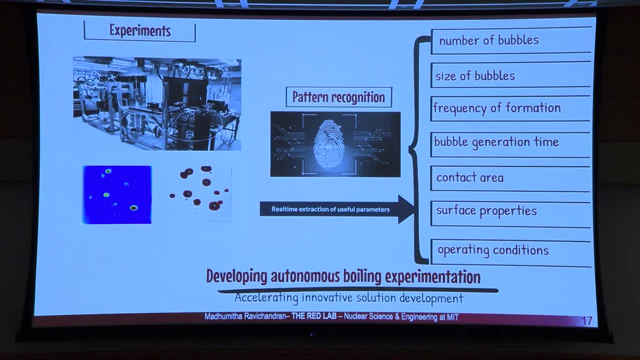 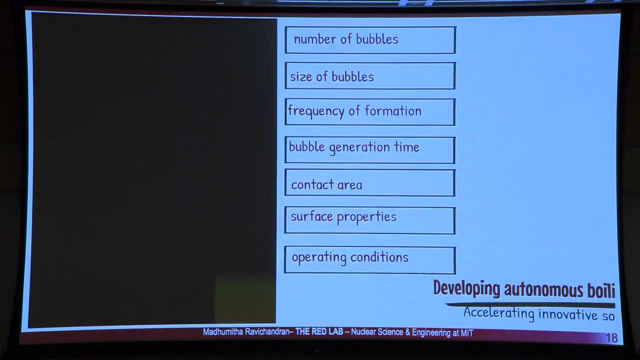 us on our experimental data and give us all the results that we need instantaneously, Like just go from the experiment to all the features that we need to determine. And, even better, what if we had a tool that would take all the features that we need to? 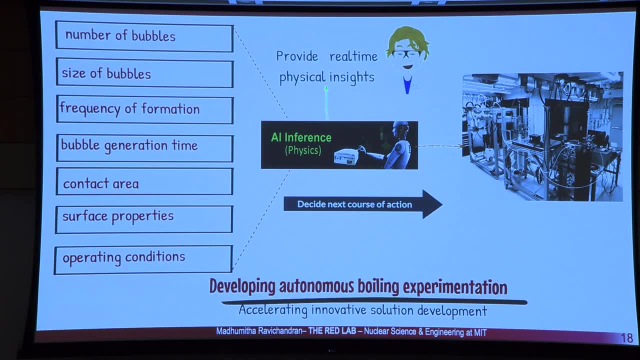 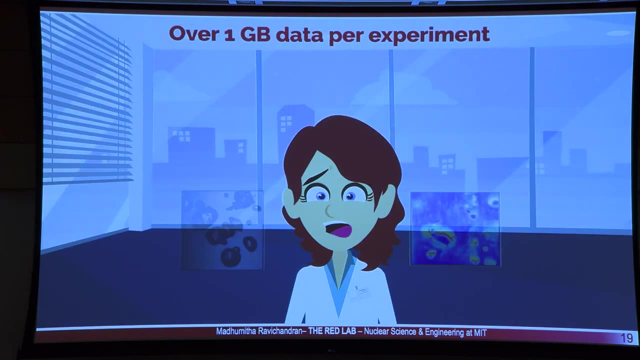 determine and make physical inferences, so that we can keep running experiments without stopping. So that was our rationale. But the data processing tool that we built should have two requirements, or satisfy two requirements, so to speak. We generate a lot of data, So from one experiment we have over a gigabyte of data. 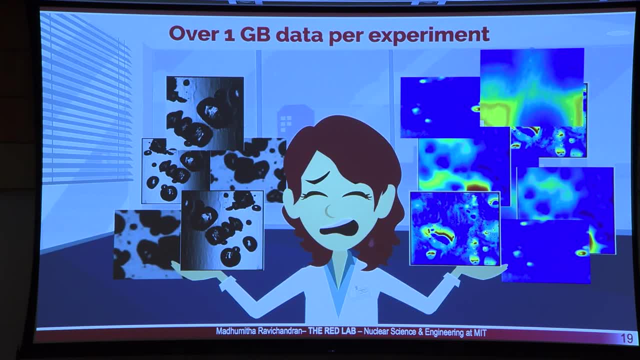 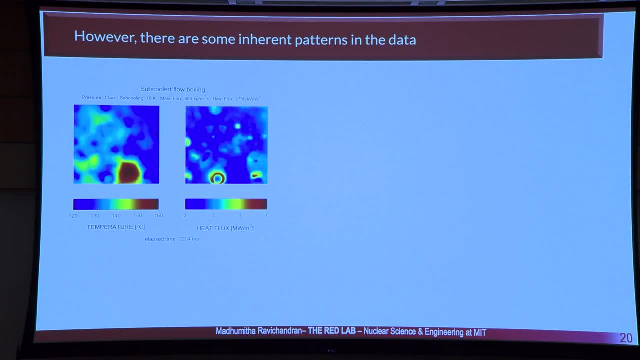 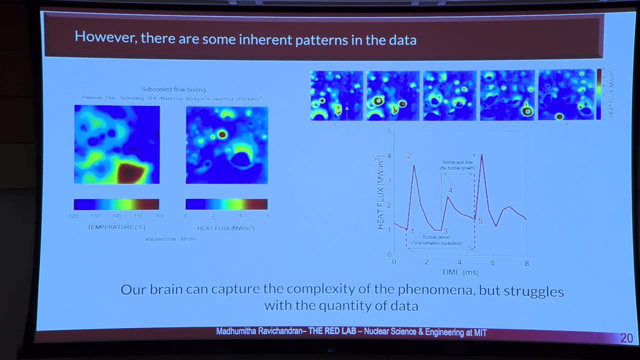 And we aim to run at least hundreds, if not thousands, of such experiments to build models. So the tool should be able to handle big data, And the other requirement is that there are inherent patterns in bubbles that nucleate and grow. If you spend a little more time, like I did with the videos on your left, you will see. 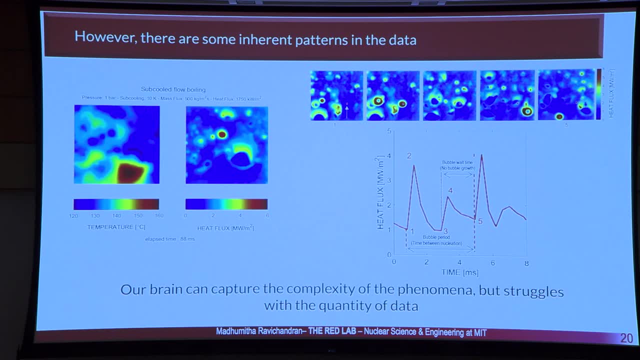 that there is a pattern to bubble growth and nucleation, as also apparent from the bubble ECGs I've plotted on the bottom right. We can all appreciate these patterns but we don't really have the bandwidth to process that data. as we see it, 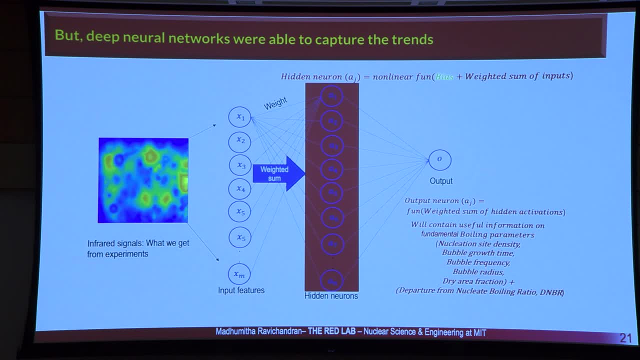 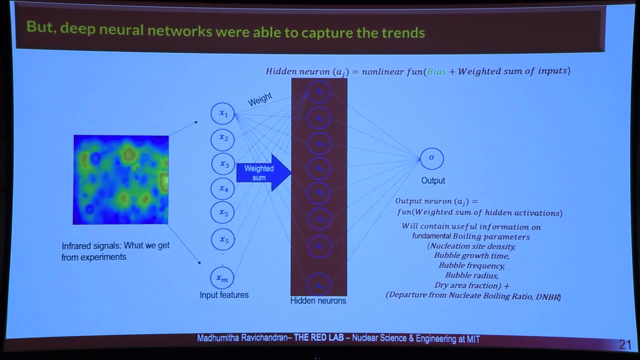 But some networks do So. deep networks have been. I mean, they were developed to work on big data. In fact, they work well only when they are fed big data, And these can take us from our inputs to the set of outputs that we need, by recognizing. 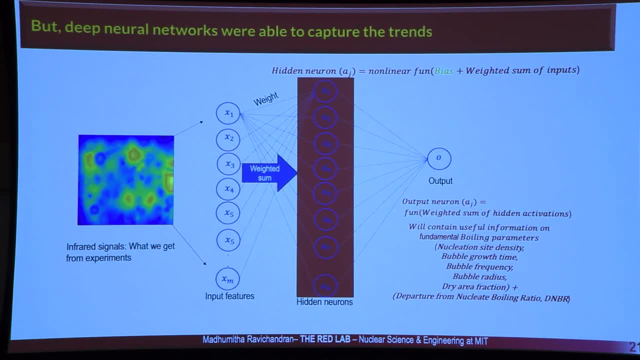 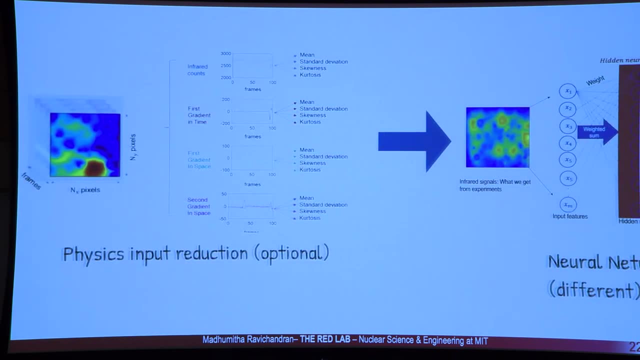 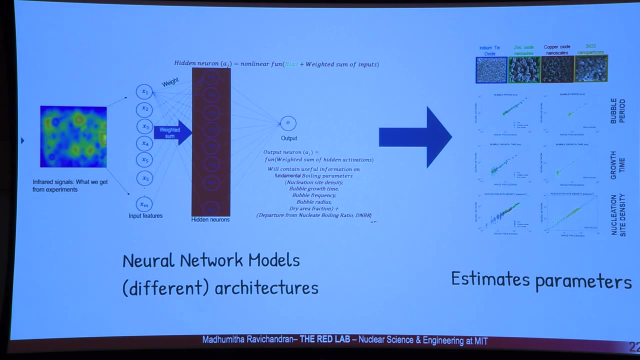 patterns- And that's widely acknowledged- of deep networks. So what we did was we ran our experiments, acquired data and fed all of these into a network that we had already trained, And this network started making patterns. It started making predictions of all the bubble features that we needed to determine. 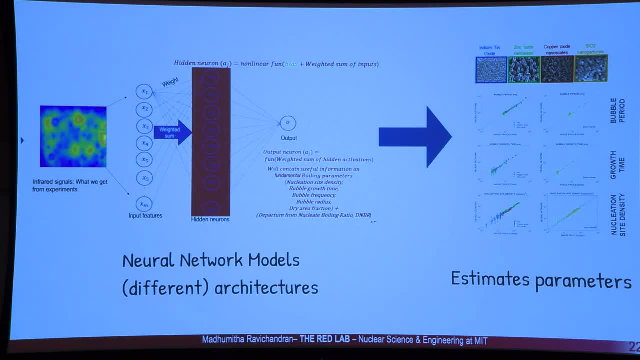 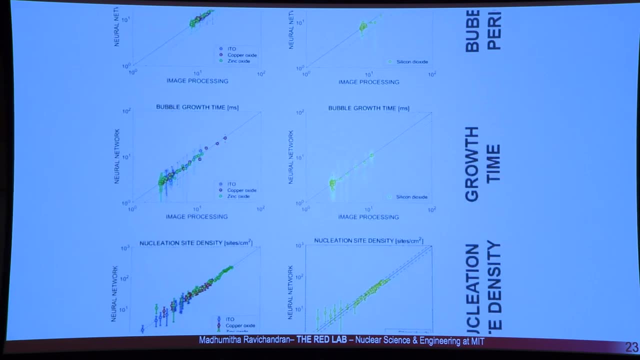 In fact, this is a bit important. If you look at it, you can see that the networks are able to make predictions for different surfaces and for different bubble parameters. So not only do we make predictions on like bubble features, like the growth time or the 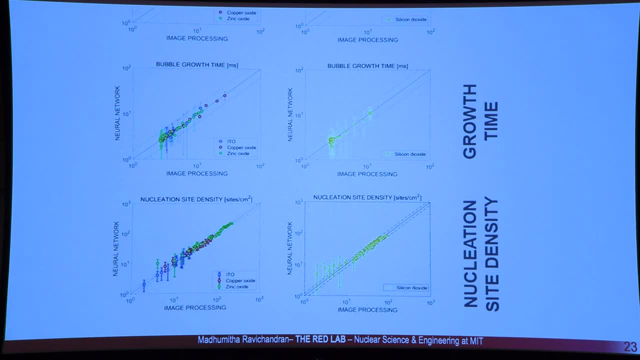 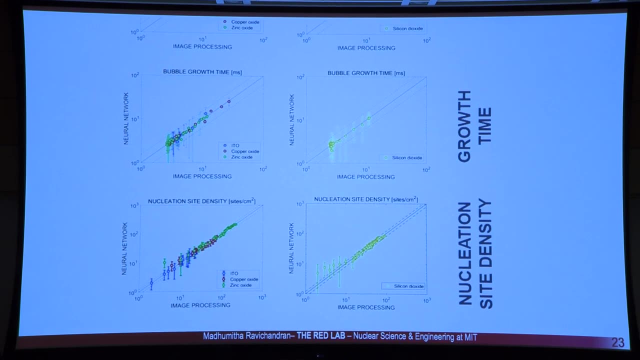 nucleation site density. but the network does so for multiple different conditions And the plots you see are the neural networks. So you can see that our neural networks performance compared with our manual post-processing tool that we've used, And you can also tell that the neural network's performance is almost on par with human post-processing. 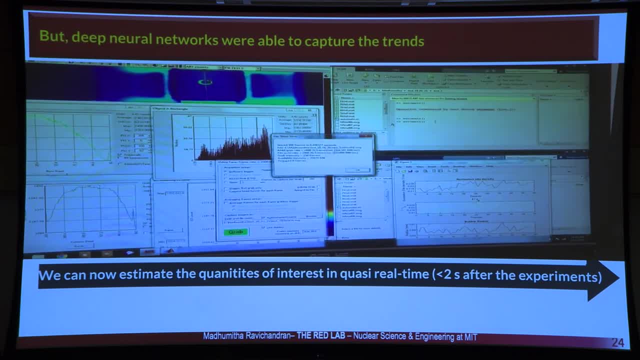 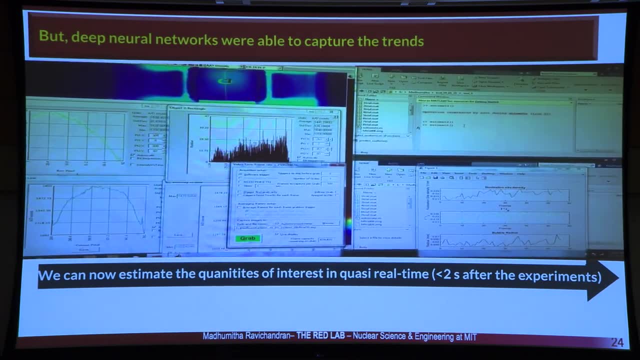 Let's make it a bit more interesting. I thought I'd show you how we run our experiments right now and acquire data So on. again, I'm not really a social blogger so I have shaky hands, But if you look at the top left you can see that that's our experimental surface over. 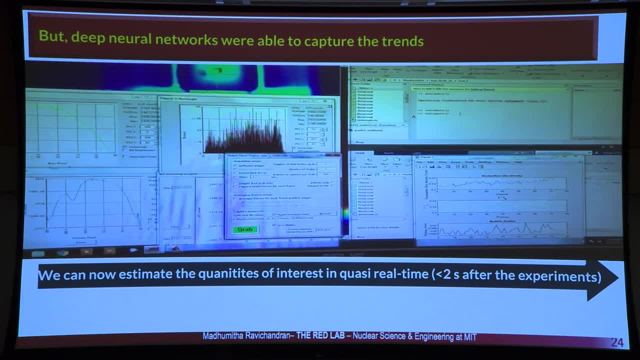 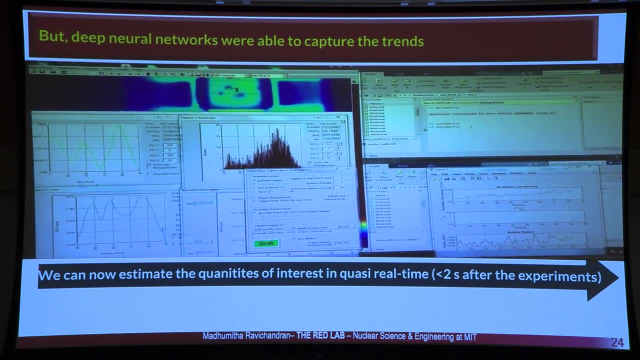 which we run experiments. You'll soon start seeing the results. You'll start seeing bubbles coming up, And on the bottom right are results for the bubble features that we want determined, And the pop-ups you see are actually the speed at which we are acquiring data and processing. 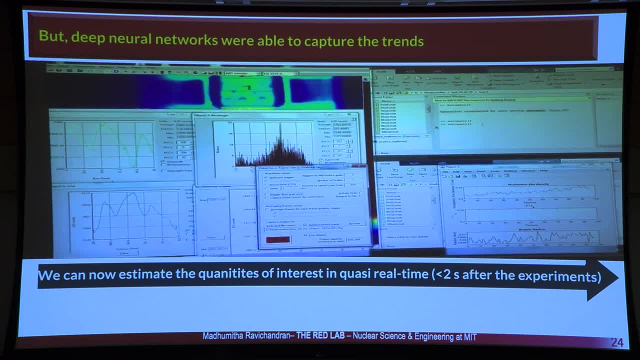 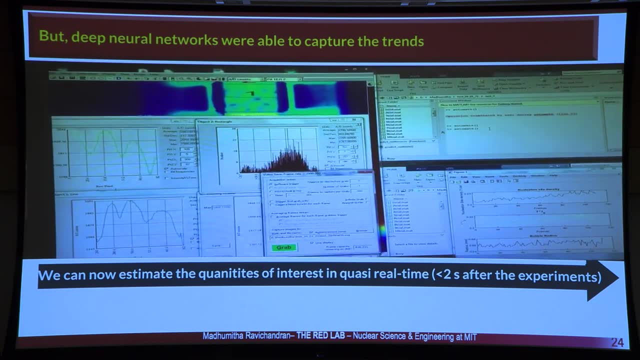 it. So let's say in one, two: yes, we've got data and we've processed it Again. So this keeps happening and it takes us less than two seconds to acquire and process all of our data And, most importantly, we also have estimates of when to expect the boiling crisis itself. 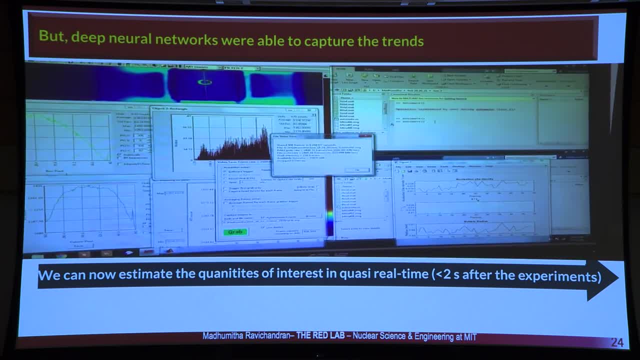 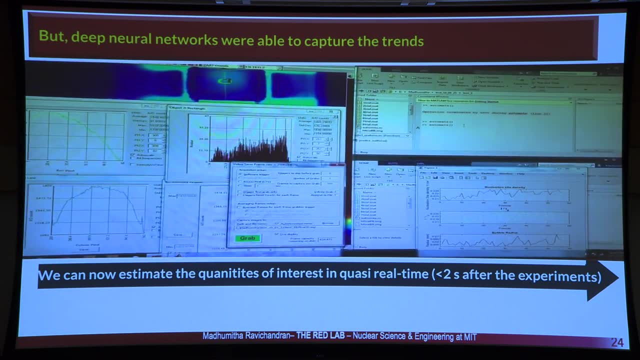 So boiling experimenters will really appreciate the fact that we don't really have to be on our toes or be extra cautious for not breaking surfaces as we run experiments, because in less than a second we might approach the boiling crisis and even break heaters. 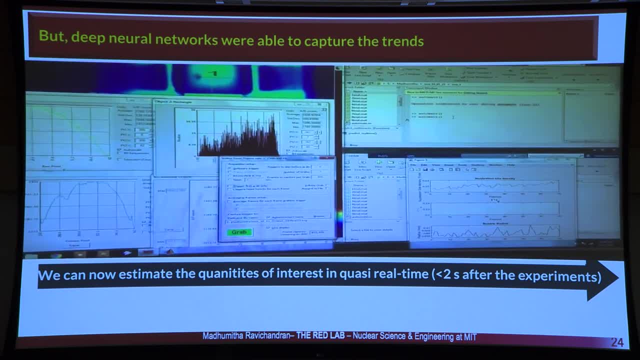 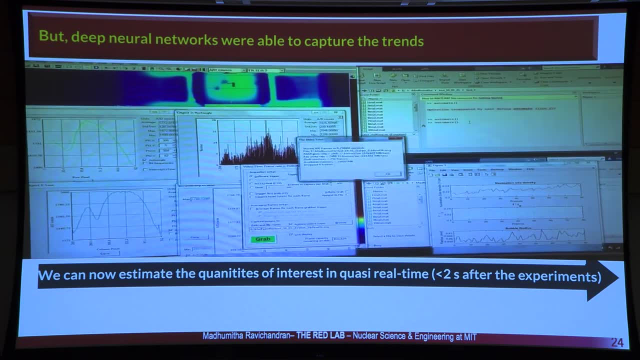 And right now we have estimates, and we might never get there Again. all the frameworks that we have built here have used MATLAB, and we even manipulate all the hardware with MATLAB. This is all well and good, But we got curious. 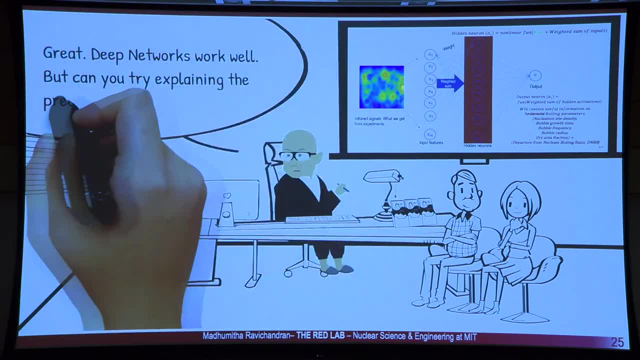 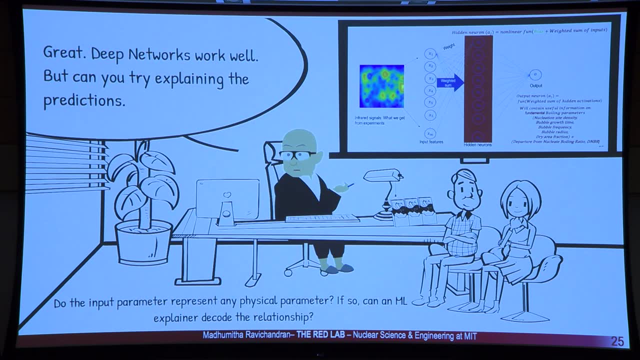 We wanted to see. We wanted to see if we could depend on these predictions and if we could believe these predictions and take them further. So for that we started questioning ourselves. We wanted to see if we could explain the predictions made by the networks that we have trained. 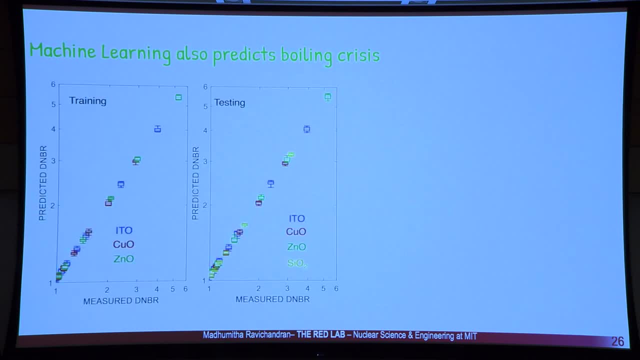 For that we chose the boiling crisis itself, because that's fairly accurately predicted by the neural networks we've developed. But we wanted to see if we could correlate the boiling crisis to some of the bubble features that we also predict. So for that we've actively monitored. 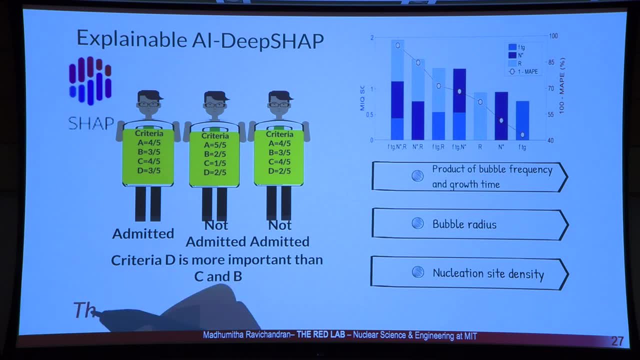 We've monitored advancements in machine learning and particularly in explainable artificial intelligence. So we've used some tools and I will show the results for DeepSharp here. So to speak about DeepSharp, I want you all to think about college admissions. 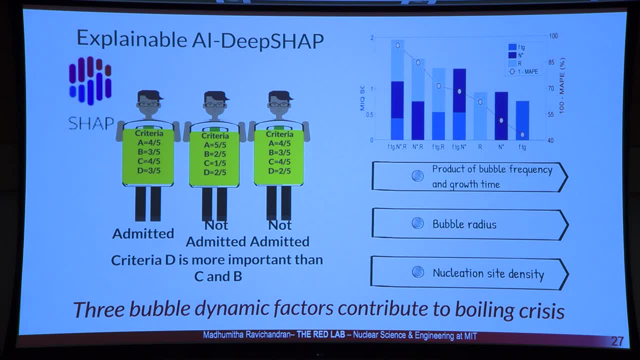 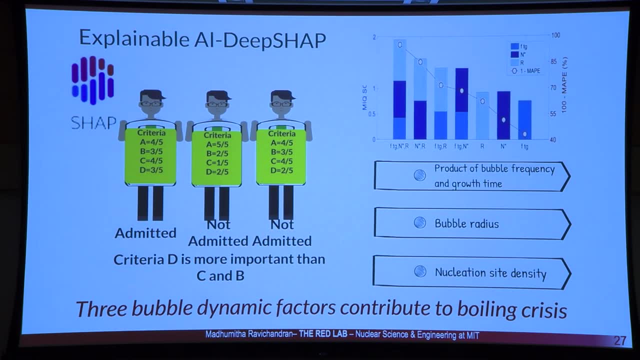 We've all been there and we've all seen the admission process. So let's say there's a pool of students and they have similar profiles, but one of them is chosen as opposed to the others, And we have these results now. 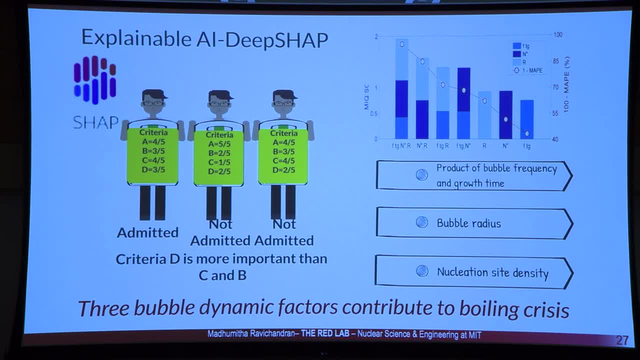 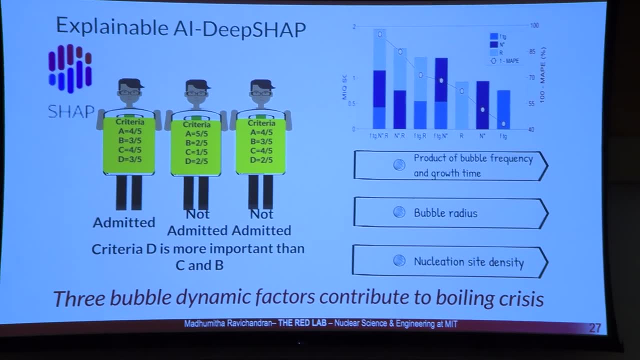 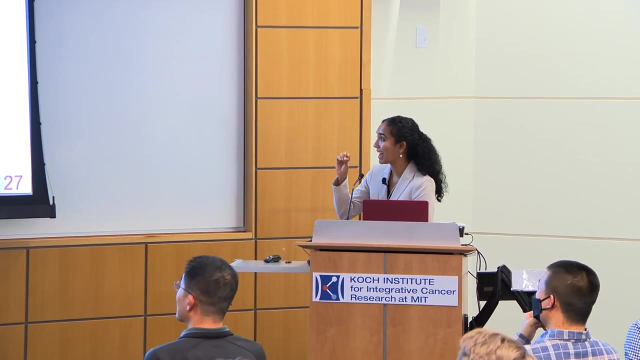 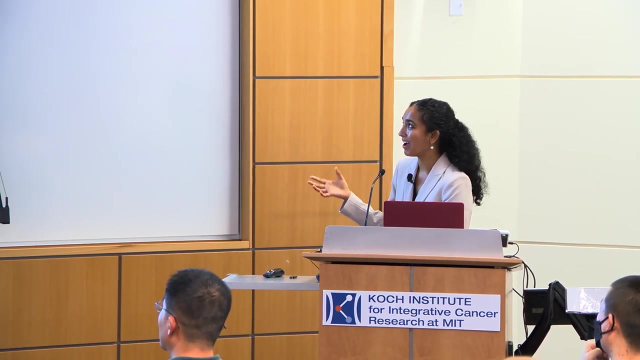 Let's backtrack, Think at what compelling factors or features that student possessed that the others didn't, And now we might be able to narrow down to what compelling factor drove a student to get admitted while the others didn't. And let's translate the same idea into the deep networks that we are training to determine. 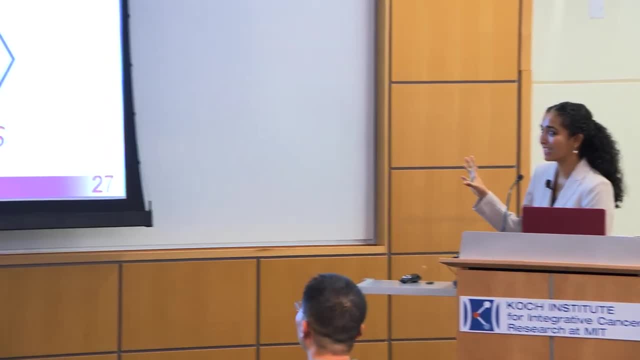 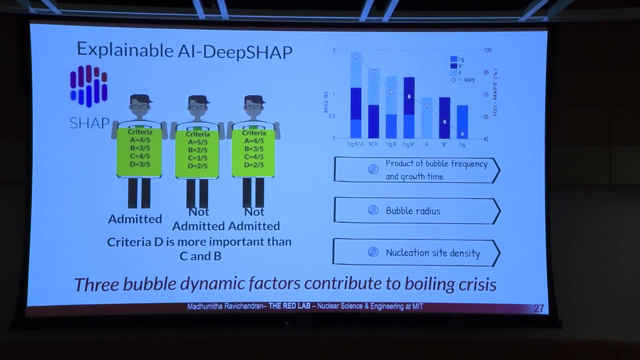 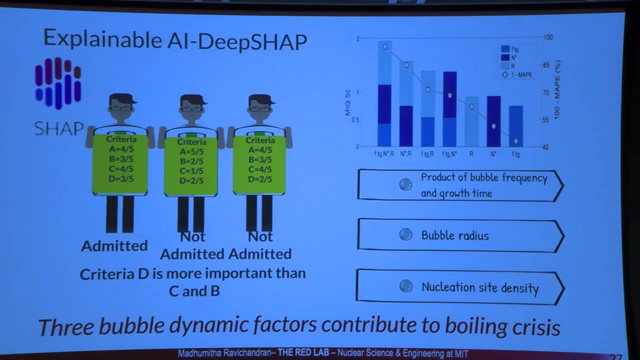 the boiling crisis, We did exactly that, but for deep networks it's a multidimensional problem and it's not as straightforward as college admissions, so to speak. Let's look at the plot on the top right. Those are the results from DeepSharp, and here we see that there are a set of features. 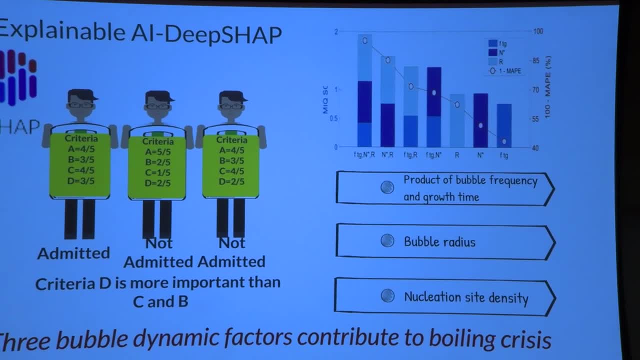 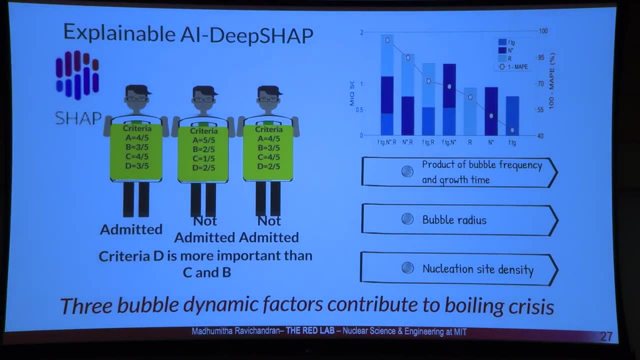 that matter the most in comparison to other features. In fact, even if we reduce some of these features, we start seeing a sharp decline in the prediction accuracy And also we start seeing a reduction in the features. So we have a set of features that matter the most. 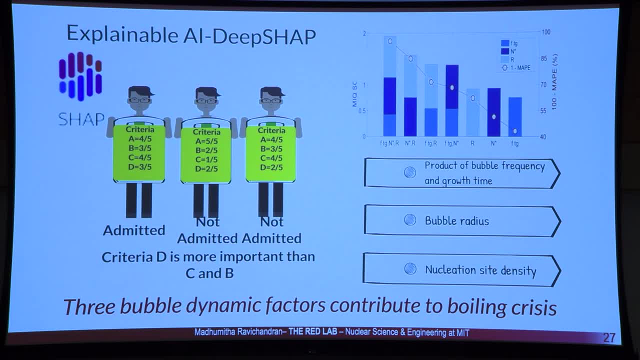 And we start seeing a sharp decline in the prediction accuracy And also we start seeing a reduction in the features And also we start seeing a reduction in the features And also we start seeing a reduction in the features And so we start seeing a reduction in the features importance itself. 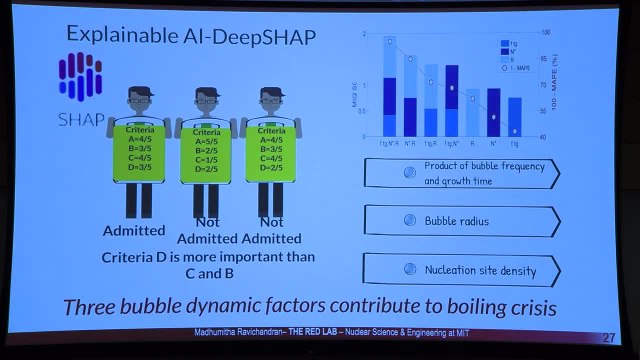 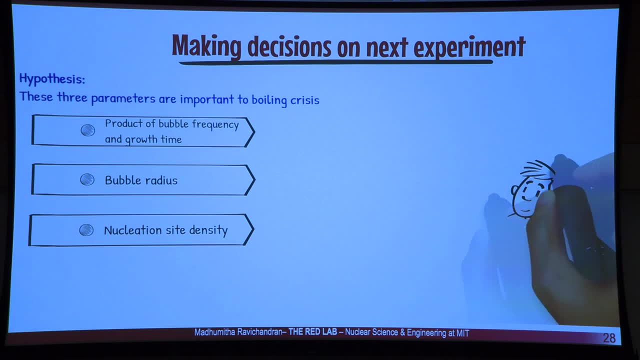 And the features that we outlined as being most important are shown beneath. So this is again. this is good, but we wanted to see, if we have this hypothesis that we say, you know, several factors impact the boiling crisis more than the others. 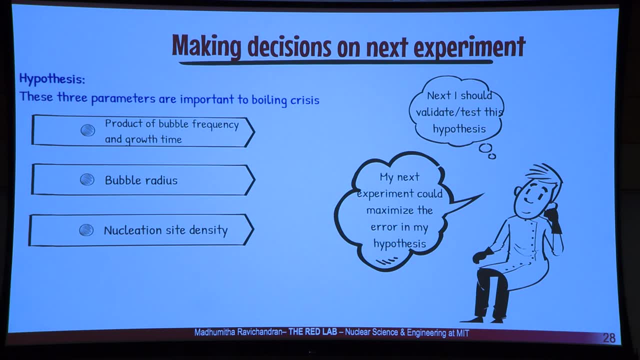 But I started thinking: how will this hypothesis break down, or where will I start seeing discrepancies, or when will other features start mattering to the boiling crisis? And to do that again, we have got the following: 1. to run a lot more experiments, to test under different conditions, and for that I thought: 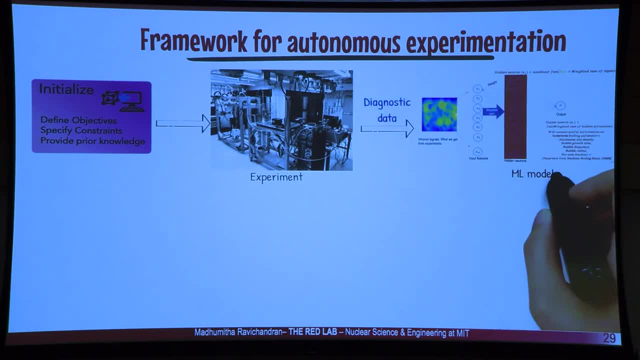 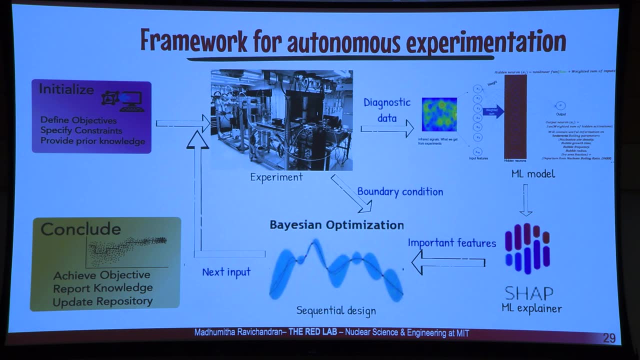 why not have a tool that, if I set it up, would start running experiments on its own- actually, that happens right now- and then have a machine learning model, tell me the results and feed those results into a deep-sharp explainer that would make inferences and the system? 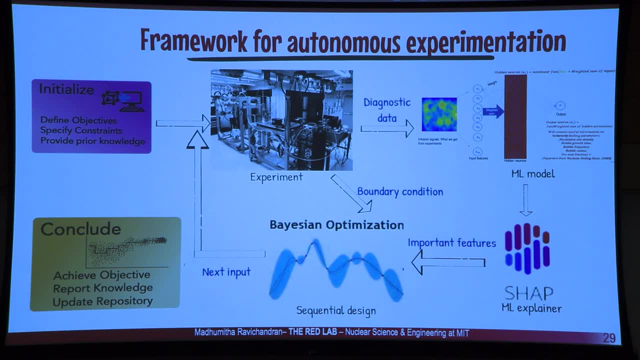 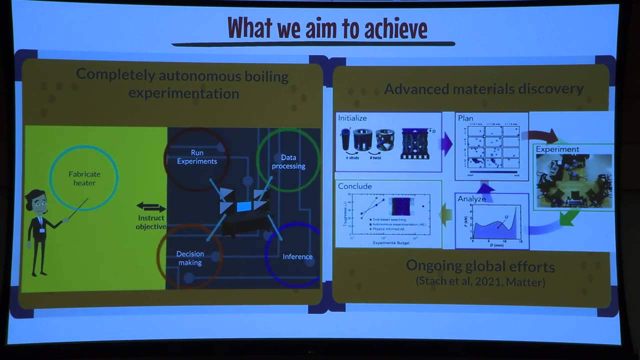 will know what decision to take, or it might even take the experiments into new conditions or new domains that we may not have even estimated. This work is again in progress. we have a few more months to complete it, but the application scope is broad. not only can autonomous experimentation be used for medicine and medical research, 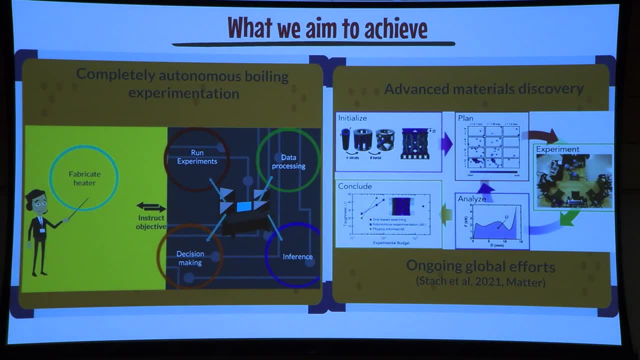 but there's another hot topic, especially of particular interest to nuclear engineers, which is advanced material discovery. that would also benefit from the use of autonomous experimentation. And I want to leave you with one thought: Okay, On boiling experimentation. imagine in a few years from now how cool it would be if. 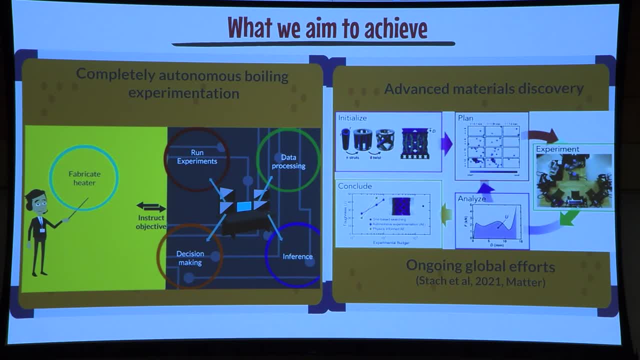 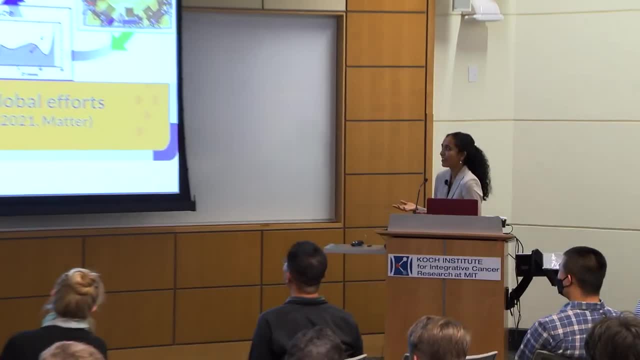 a researcher or a student only had to fabricate a heater, load it into the experiment and then they could go back home. the test section would run hundreds of experiments on its own, give inferences and also tell you the physics, and in the meantime the student could dream. 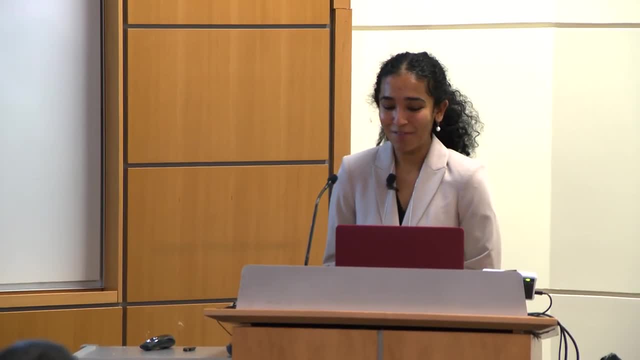 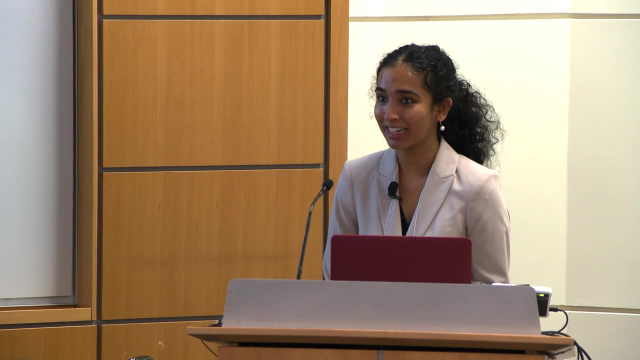 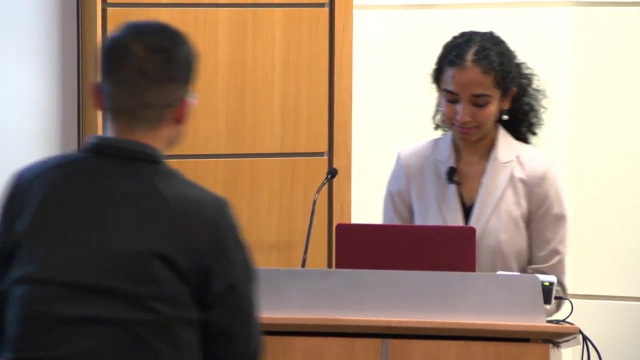 up new ideas and come up with new theories on their own. So with that, I also want to thank MATLAB for the generous fellowship that I've benefited from, and it has helped me immensely to pursue and continue my research, Thank you. Thank you, Padmita, for the wonderful presentation.